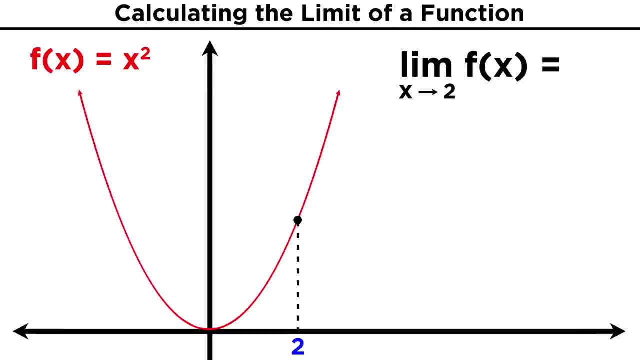 If we have f of x equals x squared and we want to find the limit as x approaches two, that will simply be four. Whether we approach from the negative direction or the positive direction, as we get closer and closer to an x value of two, we get closer and closer to a value of four for the function. 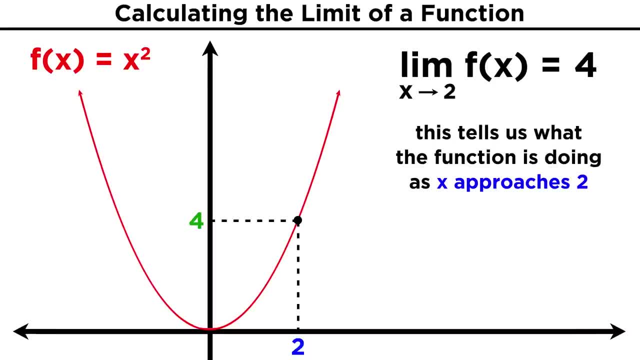 So the limit of f of x, as x approaches two, equals four. One might wonder why we don't simply evaluate the function at x equals two and get four. This is a totally valid question and in this example there is no difference. 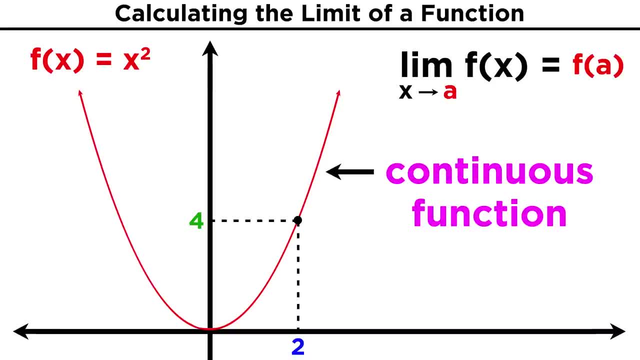 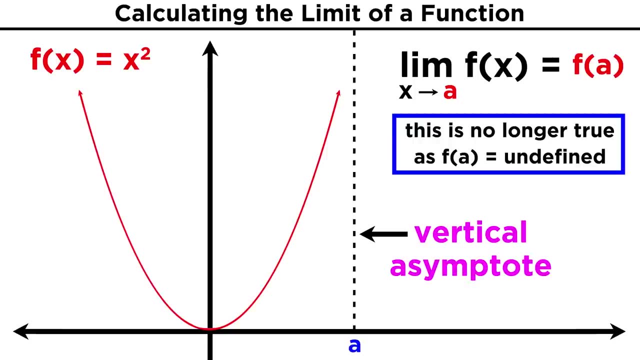 That's because this is a continuous function. The limit of the function, as x approaches a, is f of a. But some functions have vertical asymptotes and we will want to know what the limit of a function does as it approaches that asymptote from either side. but we can't just plug. 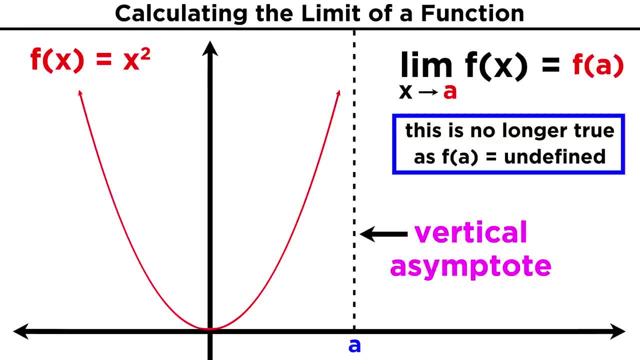 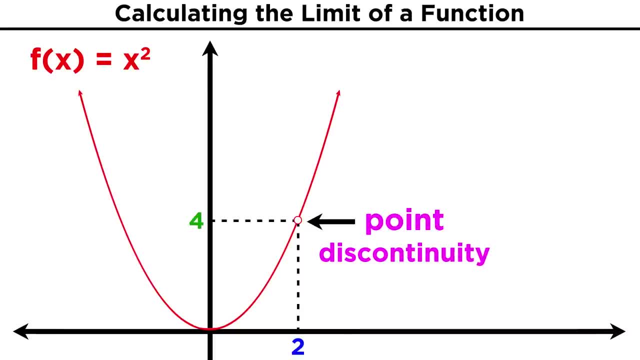 in the value where the asymptote occurs. as for that input, the function will be undefined. In other cases, perhaps, there is no asymptote, but there is a point: discontinuity. Let's remove the point from our previous example. Now, what we've described about the limit of the function as x approaches two is no. 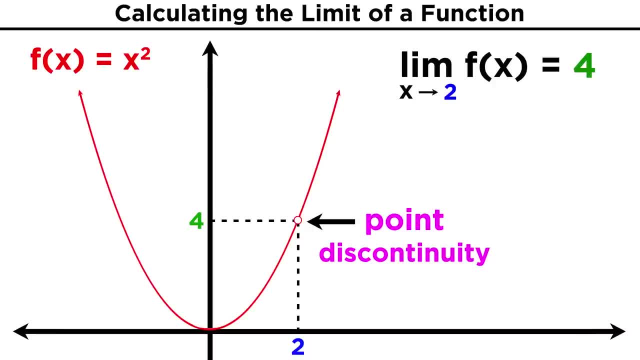 different than f of x. It's no different than what we had before, even though the function no longer equals four at x equals two. This is because the function still does the same thing as we approach two from either direction. Similarly, we may want to know about the end behavior of a function as x proceeds infinitely. 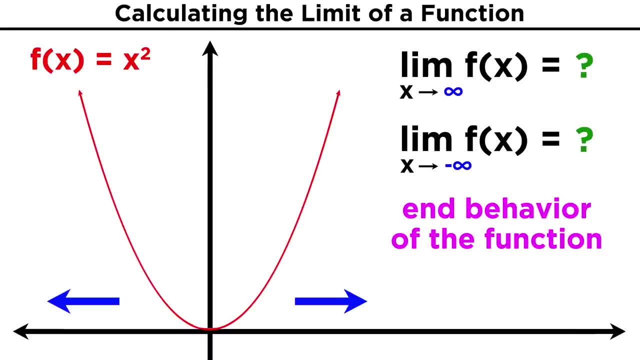 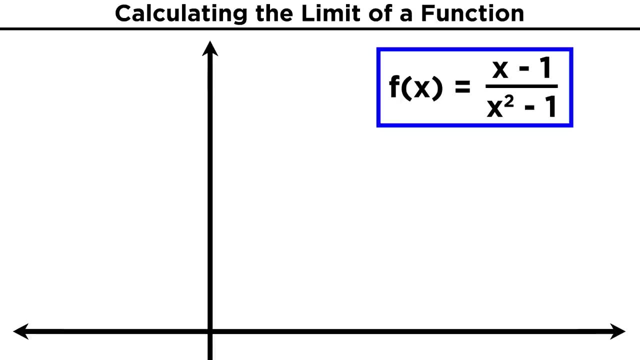 in either direction and it may not always be obvious from looking at the function in equation form. So this is the realm where limits have their application. Say, we are now looking at the function over. As we may recall from algebra, this denominator can be factored, and then this x minus one. 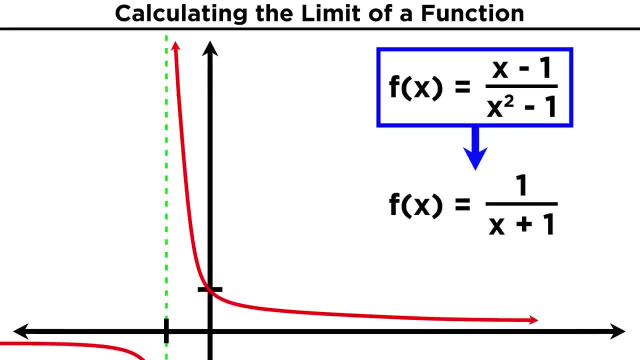 term can cancel. so this function will look exactly like one over which we can graph quite easily. But there is one difference: The original function must have a function. The original function must have a function. The original function must have a discontinuity at x equals one, because the denominator is. 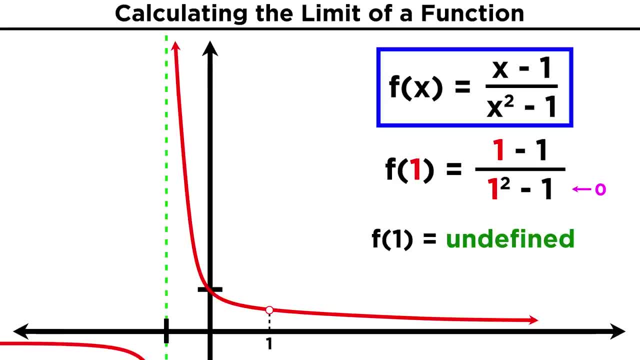 zero when x equals one, which makes the function undefined. This is an example where limits become useful, because we want to know what the function does all the way up until we get to one from either side and we can't just plug the. 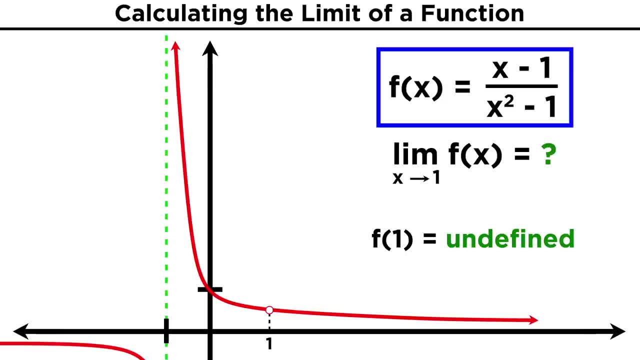 value directly into the function, like we could with the x squared function. Instead, we can plug in the function. We can plug in values that get closer and closer to one, both larger and smaller, and we can clearly see that the function approaches zero point five or one half. 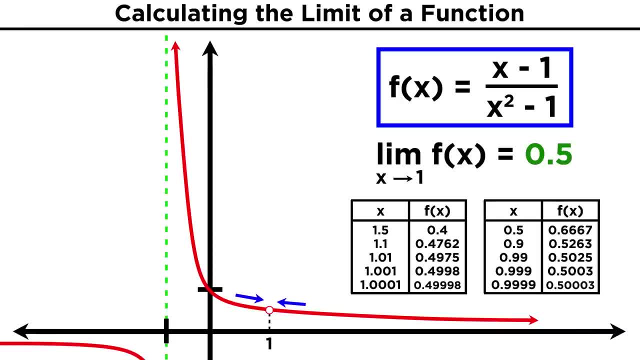 So that's the limit of this function as x approaches one. Even if we change this function so that at precisely x equals one, we give the function some other value, like two, that won't change the limit, because the limit doesn't change. 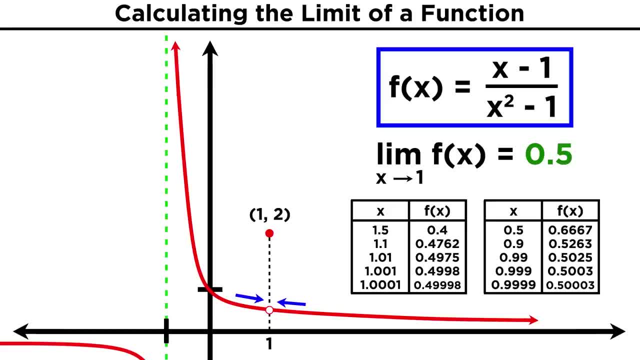 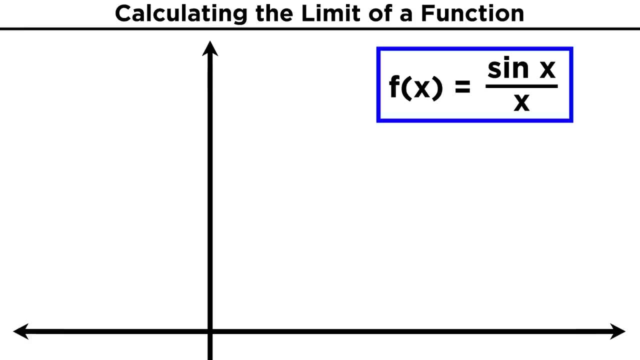 the value. It doesn't look at what the function is doing at that point, only what it is doing while approaching that point, and the behavior of the function everywhere else has remained the same. Let's look at something that would be a little tougher to graph. 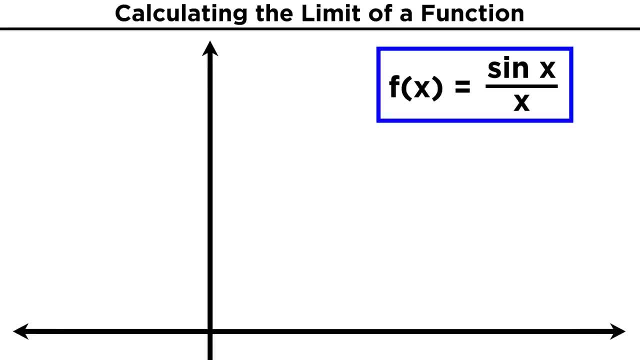 Take something like sine of x over x. What is the value of this function as x approaches zero from either direction? Well, let's plug in some numbers Now. we can't just plug in zero, because the sine of zero is zero and the denominator 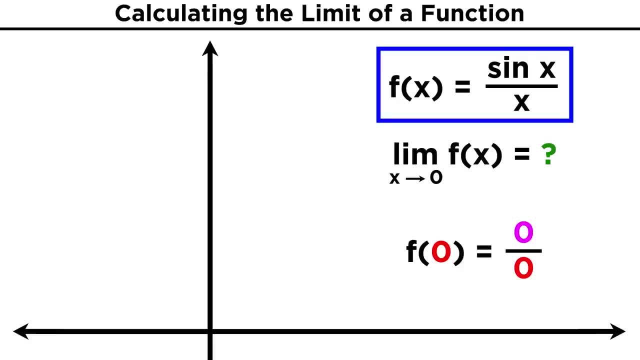 would also be zero. Having zero over zero is a big problem, because we have no idea what the function is doing at this point. from this information alone, It could be doing anything. Instead, let's plug in values approaching zero from either direction and we will see. 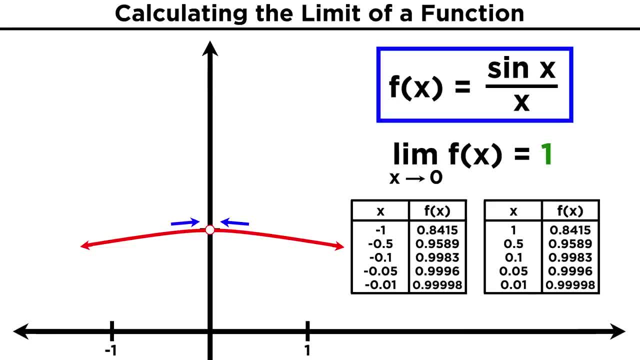 that the function is approaching one. So the limit of this function as x approaches zero is one. This is an impressive achievement because, using limits, we are able to see that something that initially looked like zero over zero was actually equal to one. so we ought to. 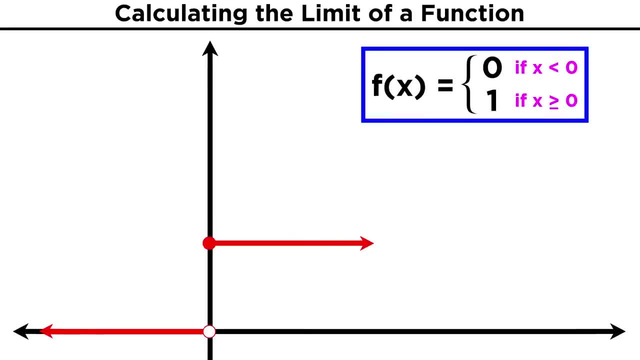 see the utility of this method. Let's also point out that the limit of a function may depend on the direction one is moving. For example, if x approaches zero, we get a different value if we are coming at zero from the positive side or negative side. so there is no limit at this value. 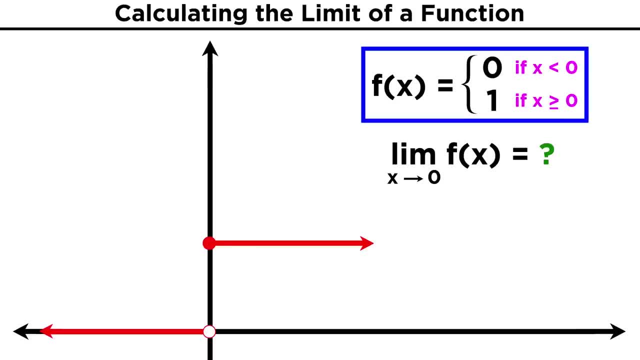 What is the limit of this function as x approaches zero? Well, we get a different value if we are coming at zero from the positive side or negative side. so there is no limit at this value, but we can instead describe two different one-sided limits. 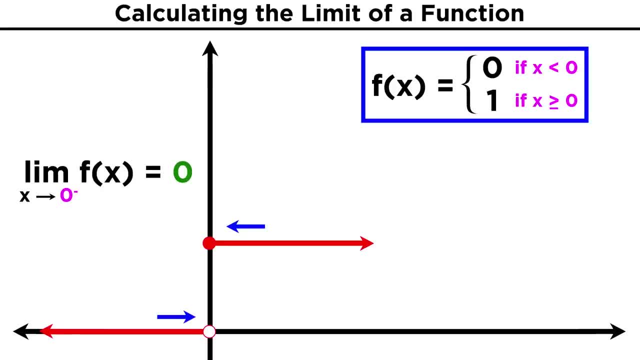 X approaches zero from the negative side, which is indicated by a negative sign in superscript over the zero is zero. We are getting closer and closer to zero, or rather, in this case, the function remains at zero. The limit of f of x as x approaches zero from the positive side, which is indicated by a. 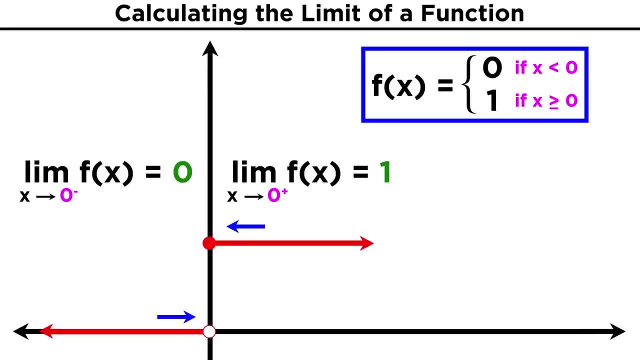 positive sign in superscript over the zero is one. We are getting closer and closer to one Or again. in this case, the function remains at one. These are called left-hand and right-hand limits. Now what about manipulating limits algebraically? 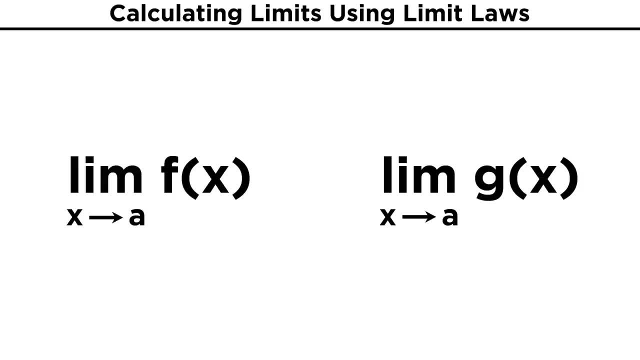 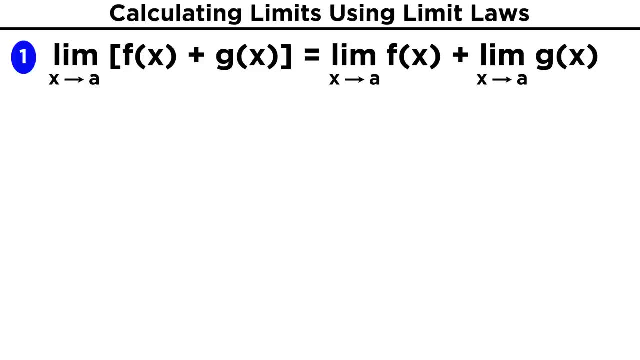 This can be done, and there are some important laws that we can learn. First, the limit of a sum of functions is equal to the sum of the limits. This should sound reasonable, as if one function approaches six and another approaches one. 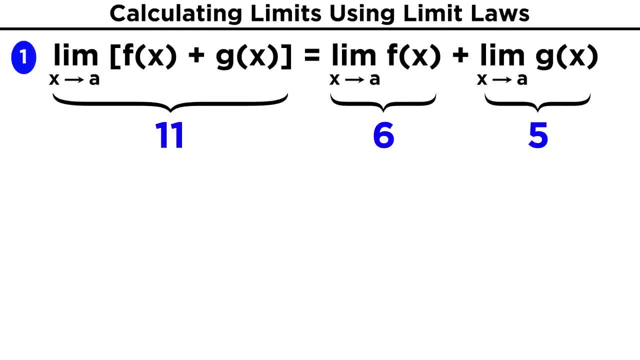 and another approaches five, then the sum of these functions should approach eleven, which is the sum of the individual limits. As obvious as this sounds, it's important to make careful sense of these things. So the limit of a sum is equal to the sum of limits. 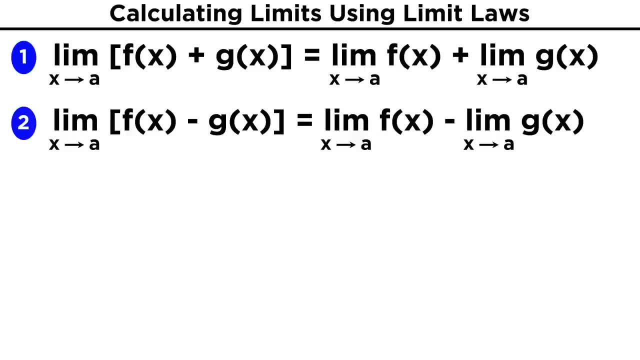 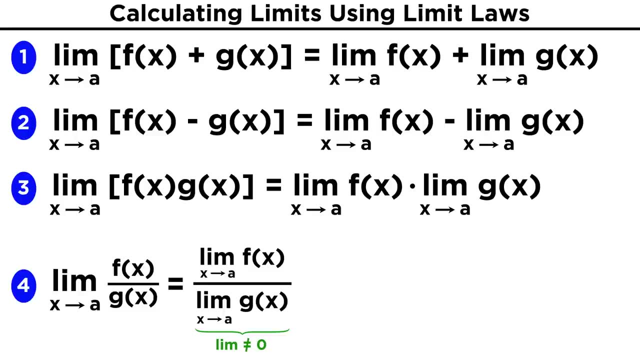 The same goes for the limit of a difference: we just switch the sign. We can also do the same thing for the limit of a product of functions, As well as a quotient, provided that the bottom limit does not equal zero. And lastly, the limit of a constant times a function equals the constant times the limit. 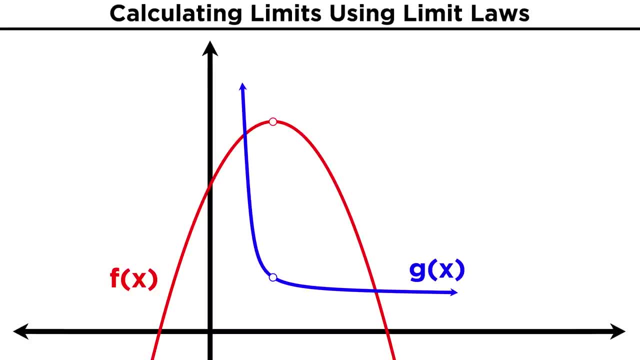 So we could look at two functions on the coordinate plane and describe particular limits at key points such as points with discontinuities. We already know how to find these limits For an individual function, So this application is no different. We are just doing algebra with limits. 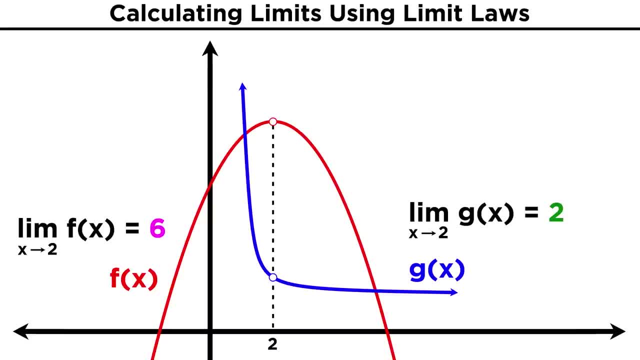 If we can find the limit of each separate function as it approaches two, then we can find the limit of f of x plus g of x as x approaches two, Or f of x minus three, g of x Or f of x times g of x. 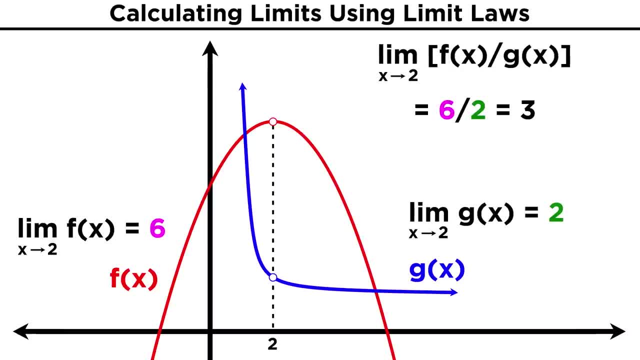 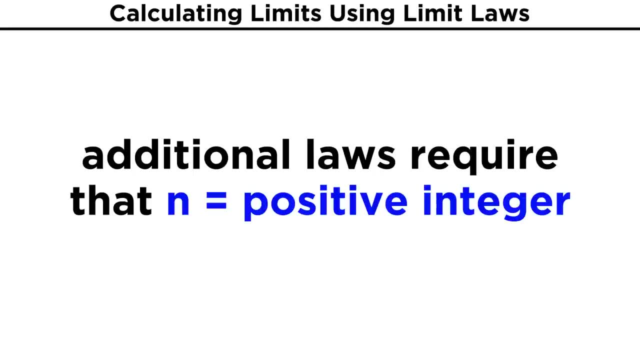 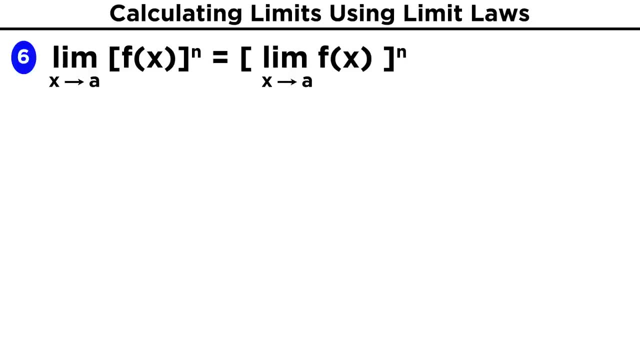 Or f of x over g of x. To these laws we can add just a couple more, all of which require that n be a positive integer. The limit of a function raised to some power, n is equal to the limit raised to that power. 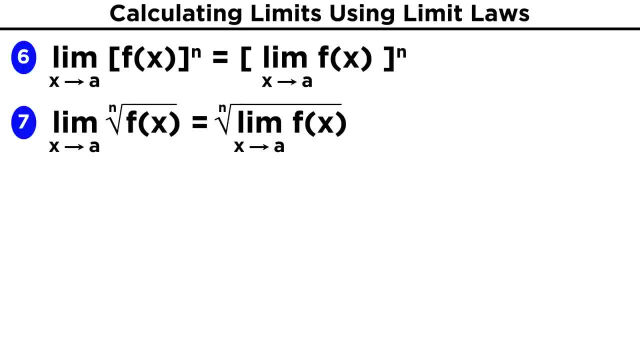 Similarly, the limit of some nth root of a function is equal to that root of the limit. The limit of x to the n, as x approaches a, is a to the n, And the limit of the nth root of x as x approaches a is the nth root of a. 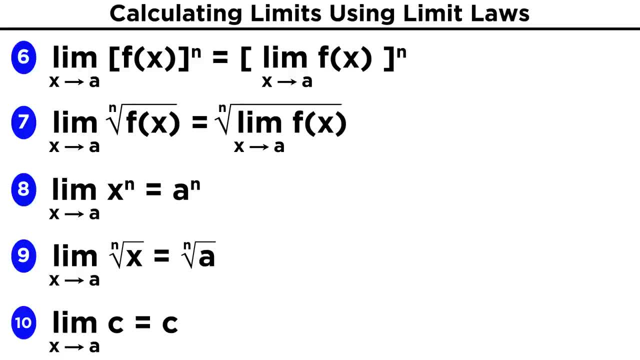 And the last two laws we will mention. the limit of a constant is equal to that constant, regardless of the parameters of the limit And the limit of x. as x approaches a particular value, is that value? That seems like a lot of laws, but they come in very handy when trying to assess the limit. 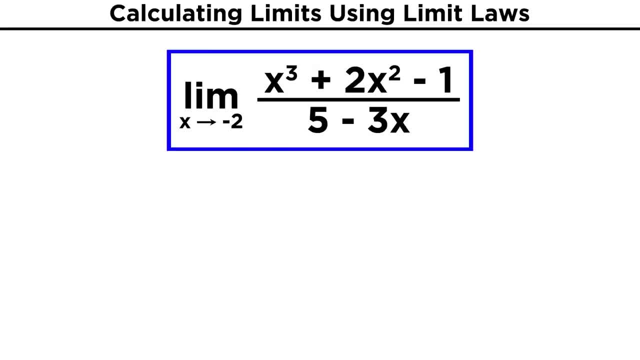 of a more complex function. Take something like x cubed plus two, x squared, minus one over five minus three x, Say we want to find the limit of this function as x approaches negative two. Now that we have these laws, We don't have to graph the function and inspect it visually, as that would take a while. 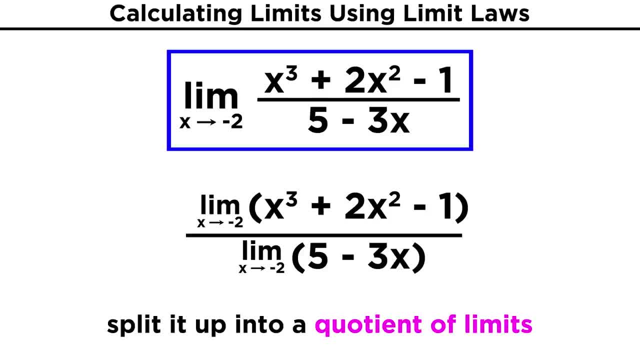 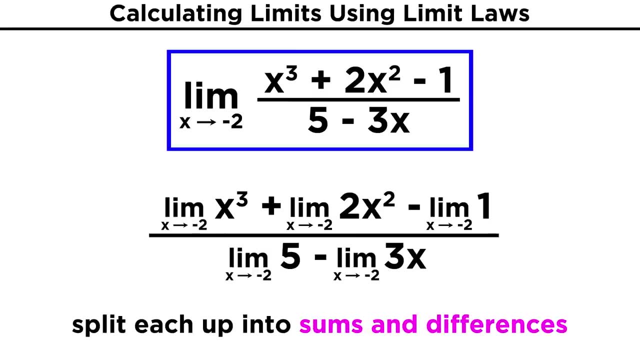 Instead, let's apply the laws. We have a quotient, so we can just evaluate the limit of the numerator and the limit of the denominator separately because of the law we know regarding quotients. Furthermore, we can split each of those up into individual terms because of the laws.